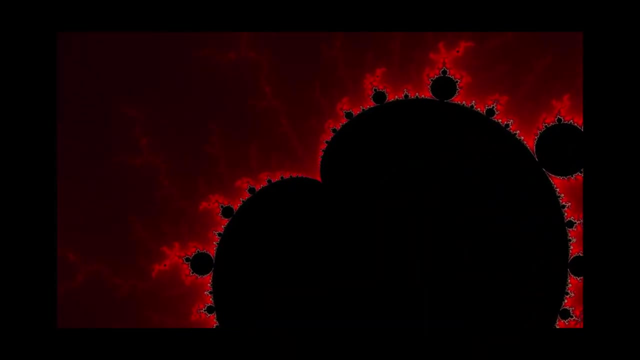 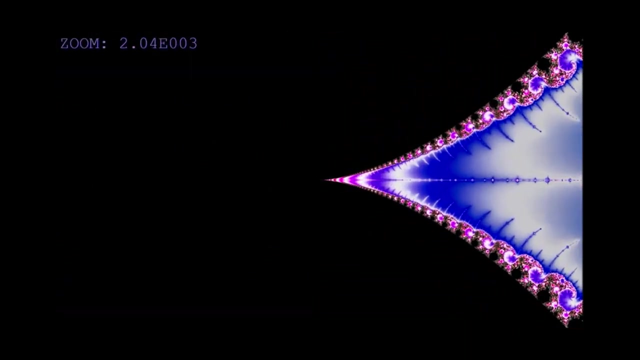 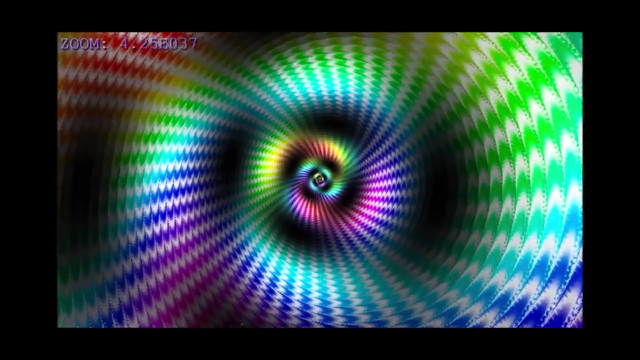 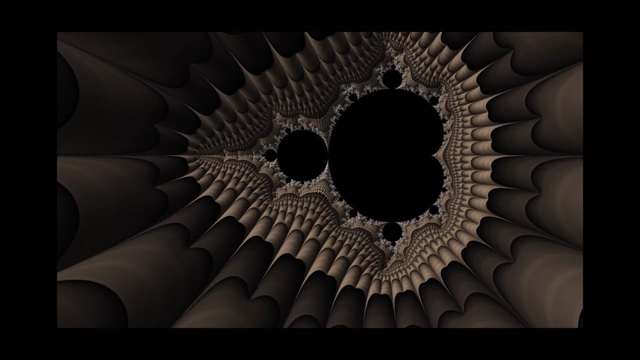 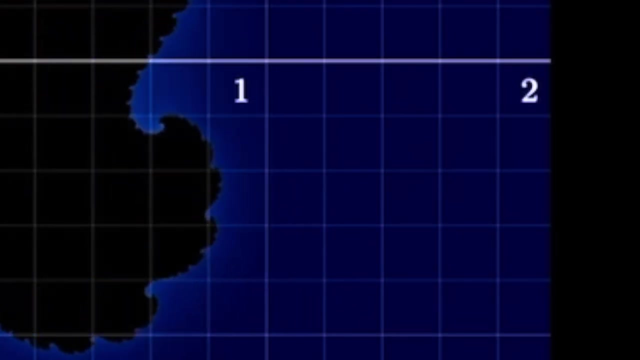 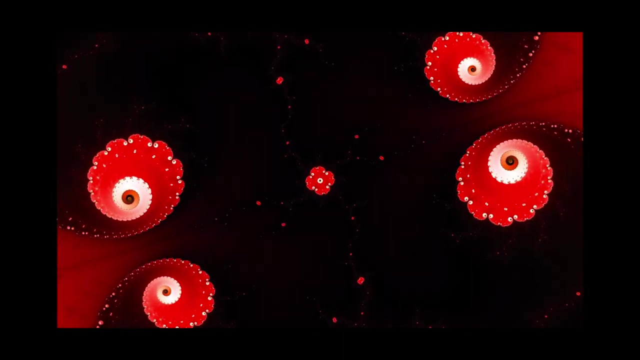 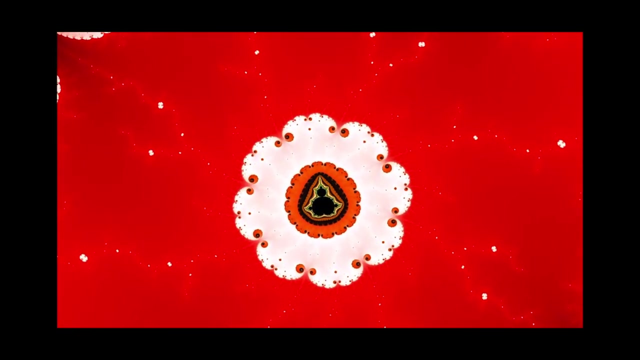 Math Numbers, What are they? For millennia, man has tried to answer this question. Numbers exist in the world around us, which led us to algebra. It took thousands of years more to then realize the math could describe a world that did not exist around us, A world beyond our. 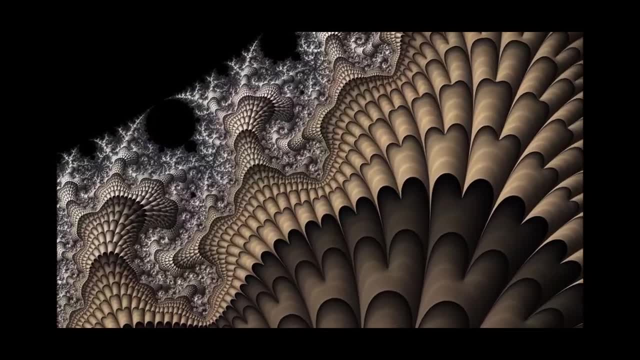 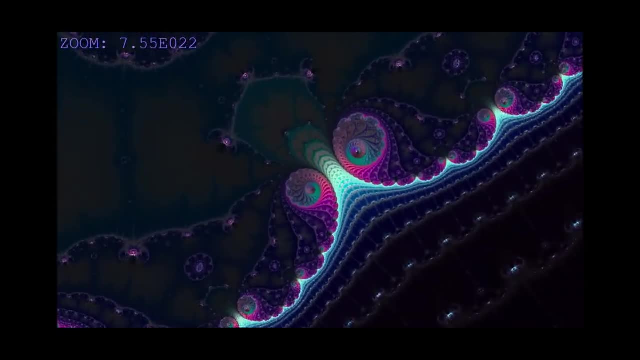 human comprehension. You've probably seen the Mandelbrot set at least once in your life, or at least heard of a fractal. What exactly is it? What does it mean? Today, I'm planning to answer that question, starting from the ground up. 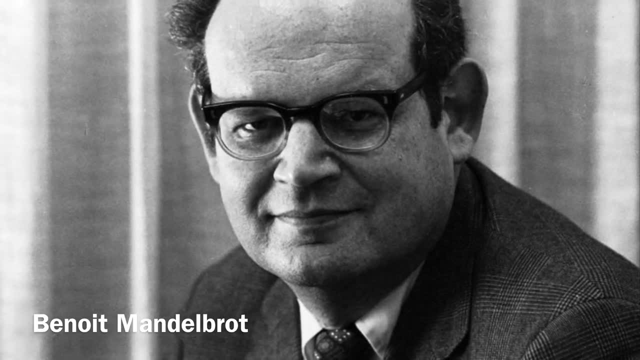 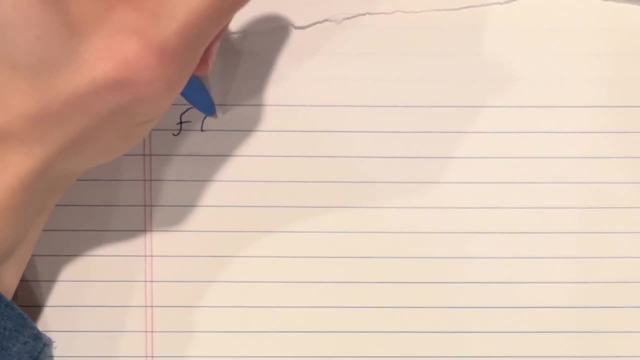 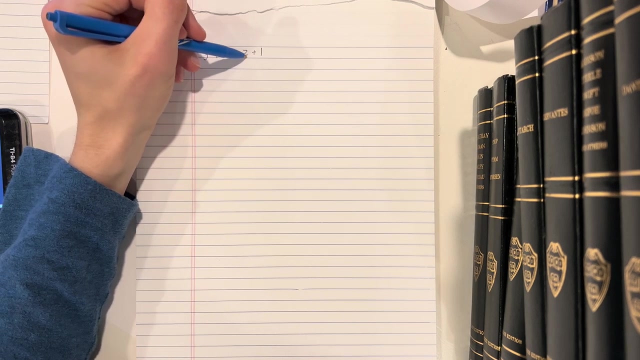 It begins with a mathematician called Bernoulli Mandelbrot, and he was studying iterative functions. Let's begin with a very easy example: f of z is equal to z plus one. This is to say, every single time we evaluate this function, we will then plug it in as the parameter, and 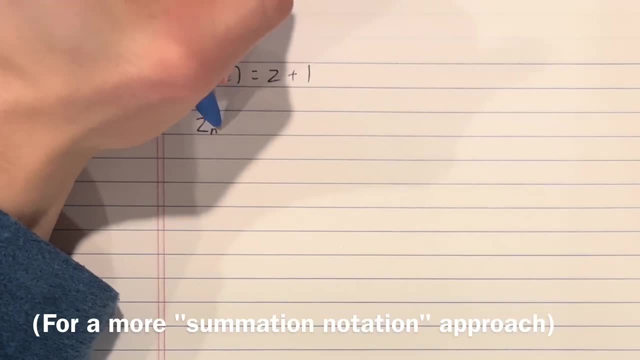 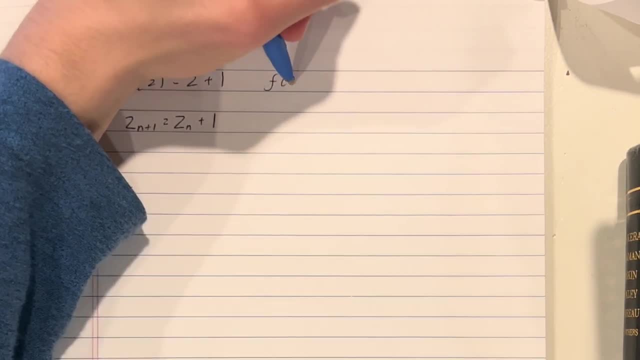 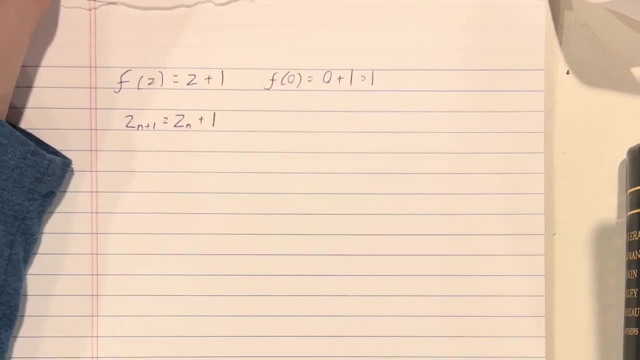 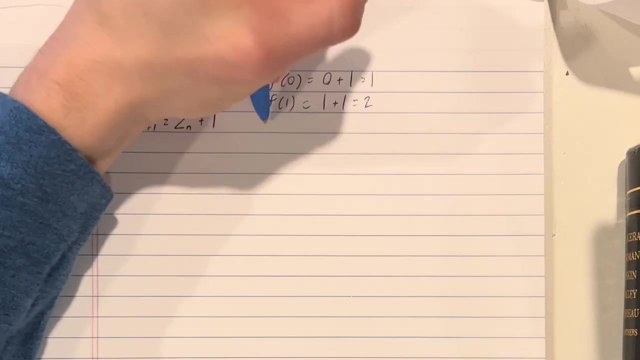 Let's start with. z equals zero. So f of zero is equal to plugging in zero for z. zero plus one, That equals one. Now we will evaluate f of one. Plug that in for z again. One plus one is two. Now we will evaluate f of two. The pattern is: I evaluate the function and 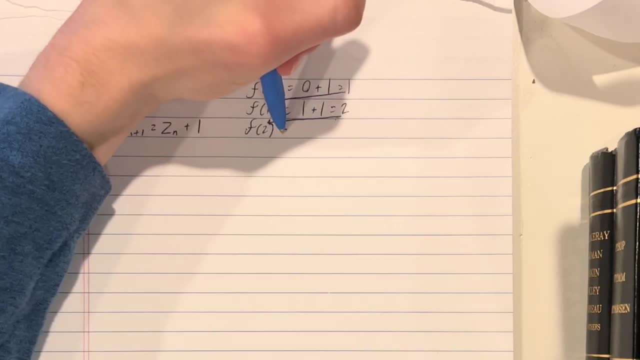 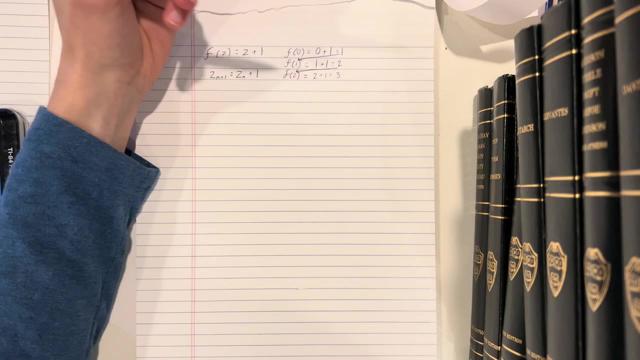 then I plug it in and evaluate the function again. f of two is two plus one equals three, Etc. This one is quite easy to see the pattern: It's just increasing by one each time. I'd made this one instead, maybe a plus two, and it would increase by two each time. Three: 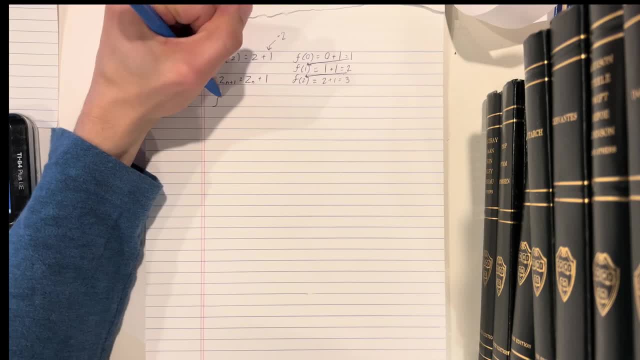 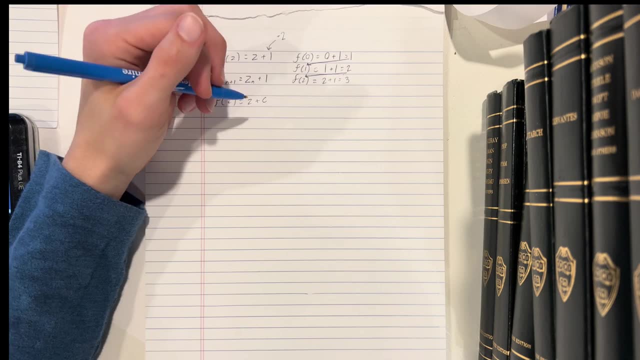 would be a three increase, and so on. Another way we could write this function is: just f of z is equal to z plus c, c being some constant. Seems simple enough, right? Mandelbrot, however, took this one step further. 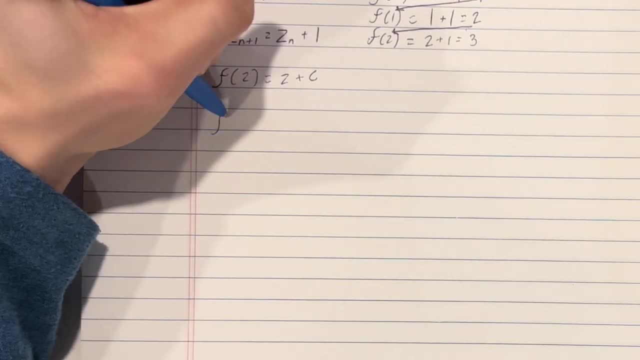 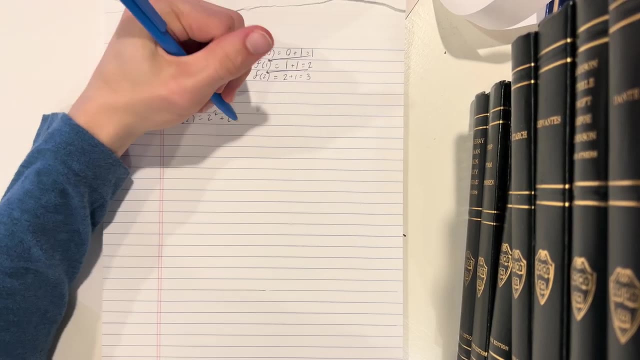 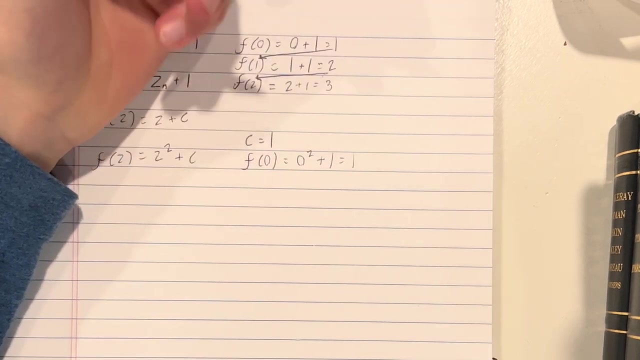 The function that Mandelbrot is studying is: f of z is equal to z squared plus c. Once again, let's just choose the easiest example and let's say c is equal to one. So f of zero is equal to zero squared plus one, which is one. F of one is equal to one squared plus. 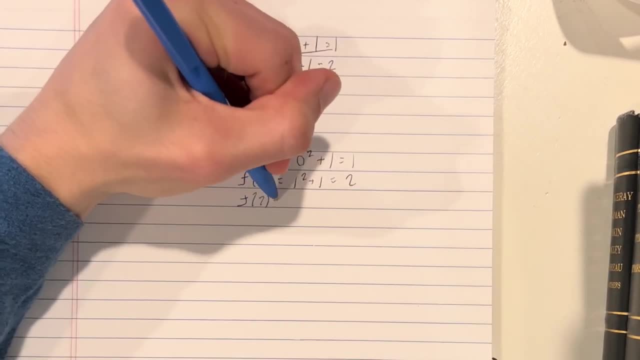 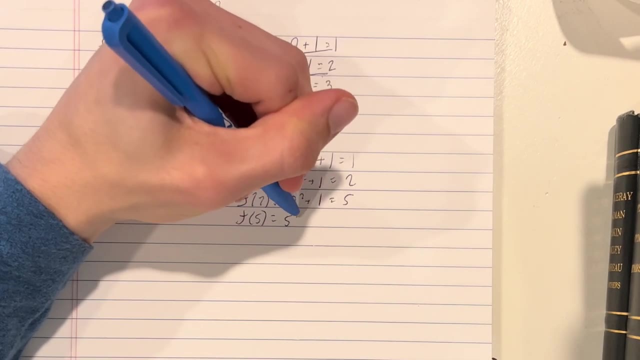 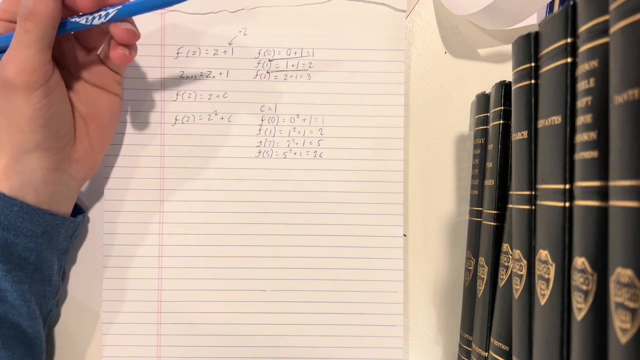 one which is two. F of two is equal to two squared plus one which is five. So f of five is equal to five squared plus one, and this is twenty-six. It should be pretty obvious that this time it is just going to quickly spiral out of control and diverge to infinity. 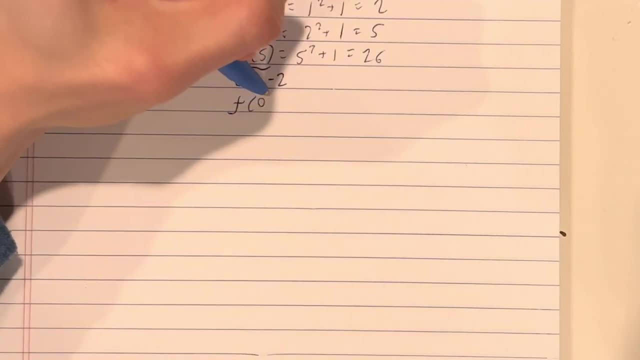 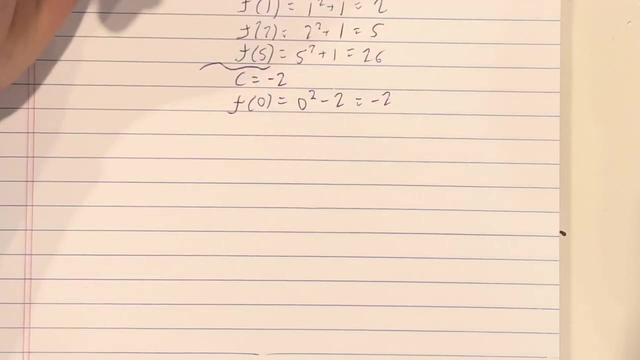 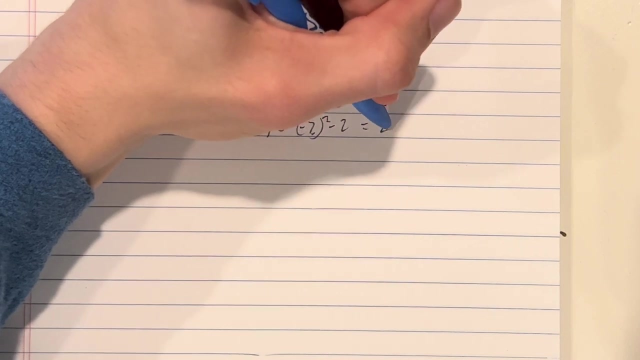 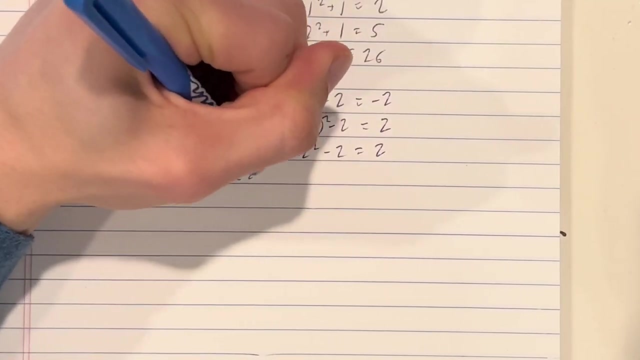 But now let's try plugging in negative. two F of zero is equal to zero, squared minus two, this time, which is equal to negative two F of negative two is equal to negative. two squared minus two, It's just positive. two F of two is equal to two squared minus two, which is two. Wait, this will just continuously. 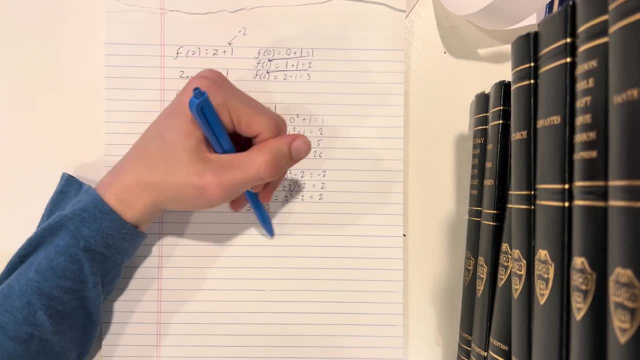 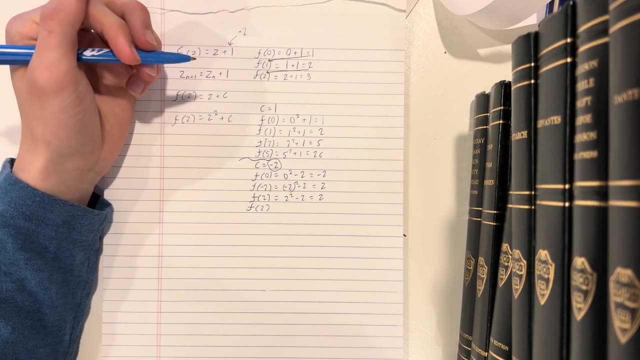 get two, plug in f of two, get two again, and it will repeat this for infinity. That means that negative two is on the boundary of the Mandelbrot set. I've drawn a number line to illustrate this concept. Negative two is the largest magnitude. 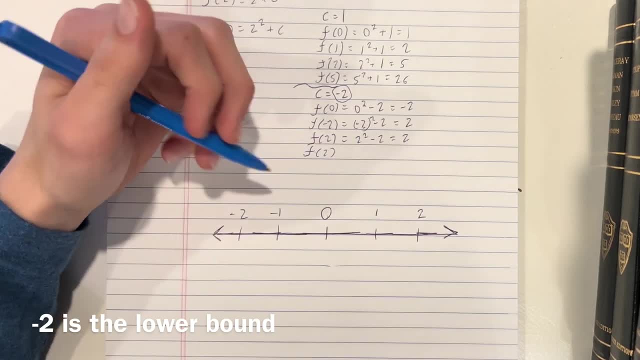 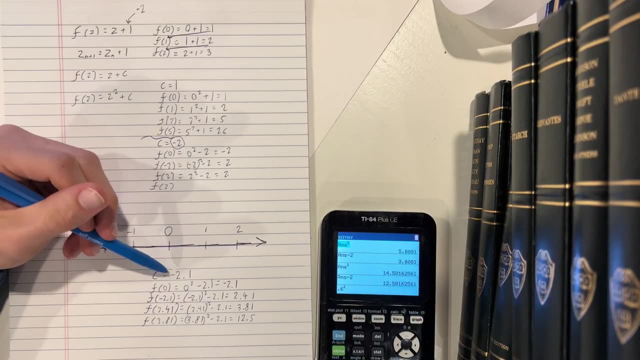 number that you can stray away from zero, such that it does not just diverge to infinity. If you don't believe me, let's try plugging in negative two point one. As you can see here, when we use negative two point one for C, we go from negative two point one two. 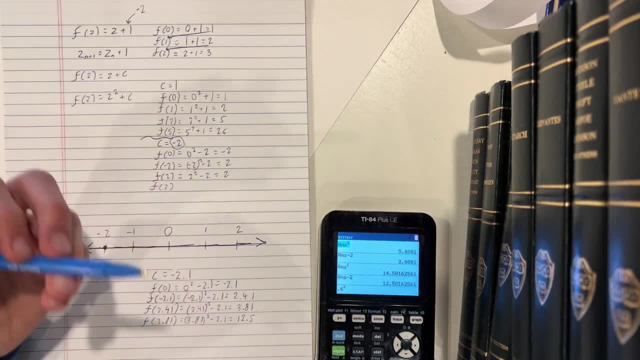 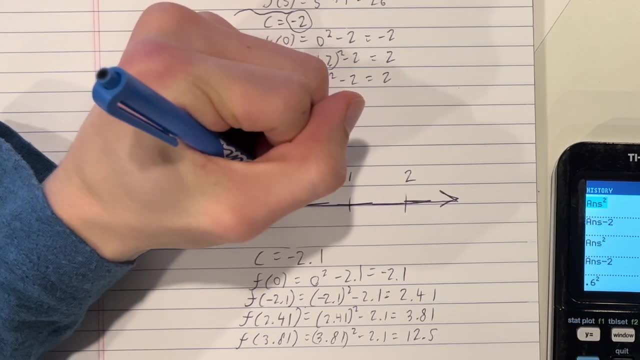 point four, one three, point eight, one twelve, point five, and then it will just keep getting exponentially greater. So we know that the Mandelbrot set is bounded by negative two. If you're curious, what the positive boundary is is actually one. fourth, and this is actually 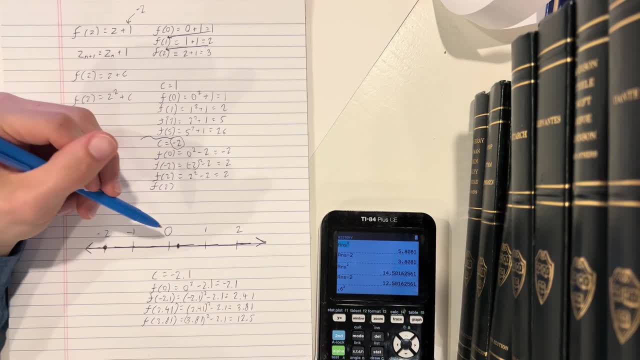 not as intuitive. When you plug in one fourth for C, then you will just keep getting a number that is closer and closer to one-half. This is actually not as intuitive. When you plug in one fourth for C, then you will just keep getting a number that is closer and closer. 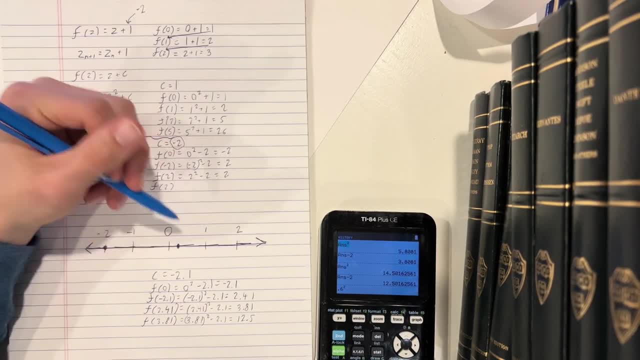 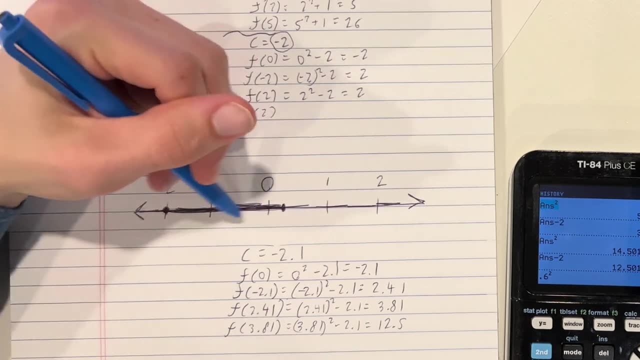 to one-half, but never quite there. Anything greater than one-fourth and we will spiral off into infinity. We can draw a bit of a shaded region connecting them, showing that the Mandelbrot set for real numbers is all the numbers between negative two and positive one-fourth, Some people would 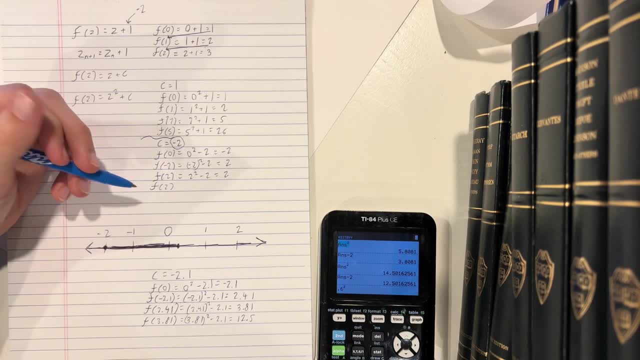 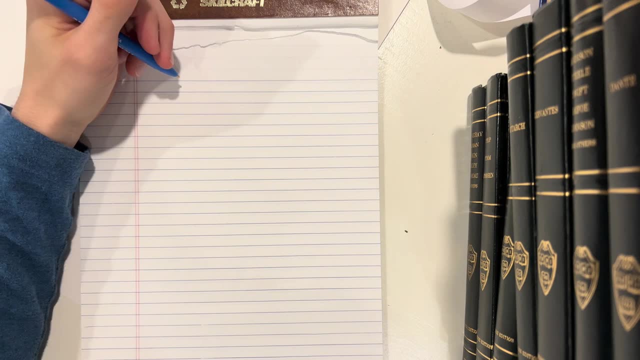 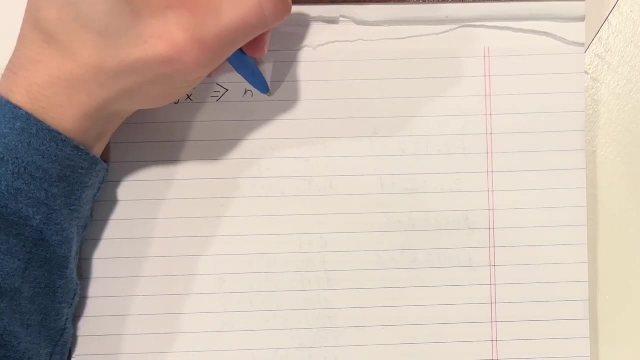 have stopped there, but what happens next is about to get a little bit more… complex. If you don't know what imaginary numbers are, it's okay, I'll run through them really quickly. Square root function. Square root function tells me a number times itself. that will give. 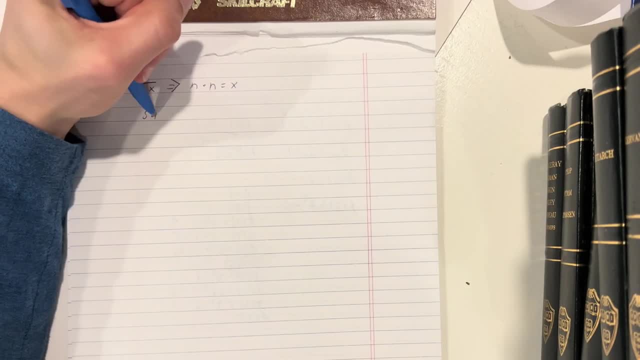 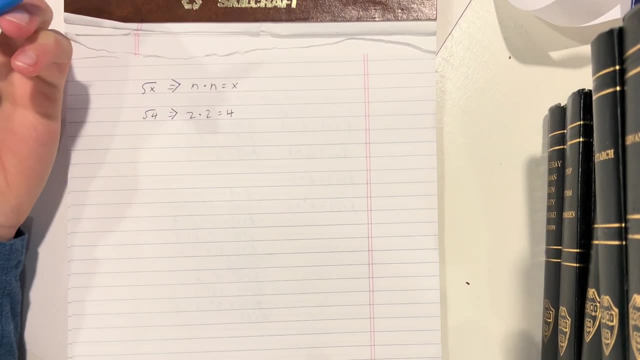 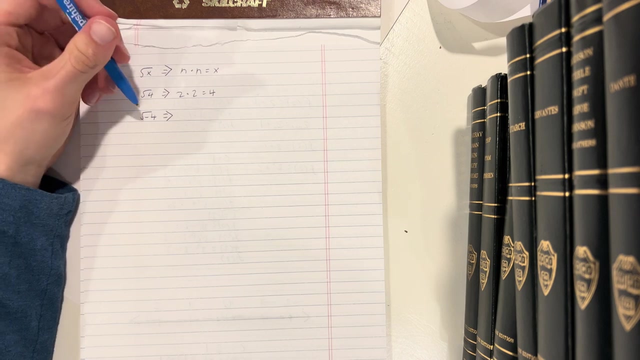 me my number under the radical. So, for example, if I had the square root of four, that is telling me that since two times itself is four, the square root of four is two. But what if we had something like the square root of negative four? Can you tell me a number? 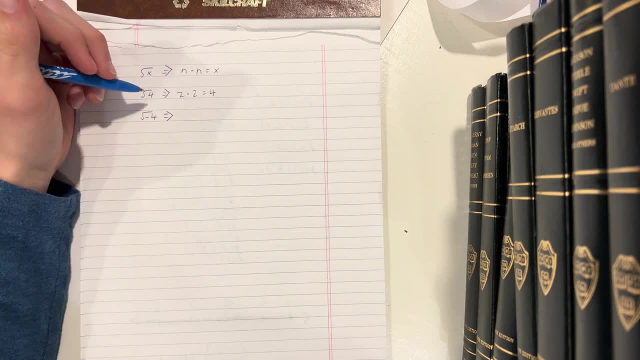 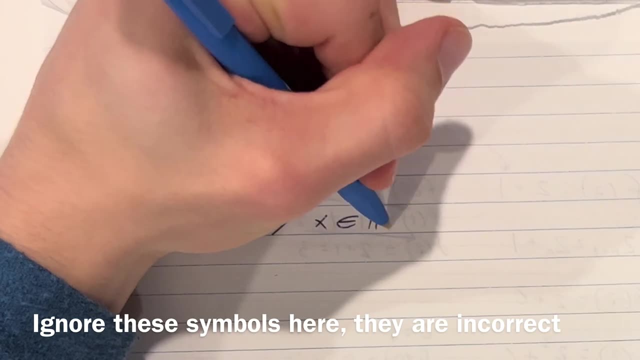 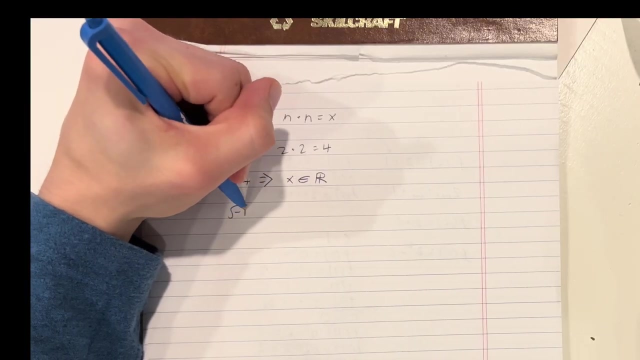 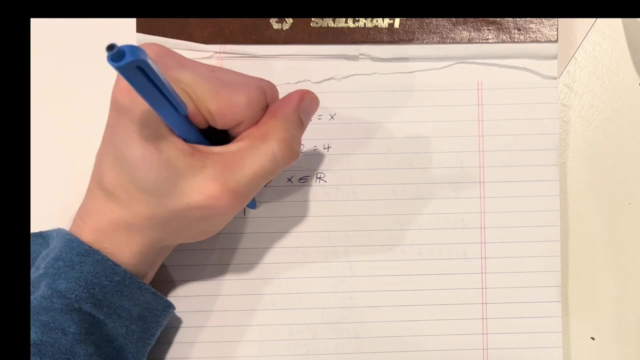 multiplied by itself, that will give you negative four. You can't, And that's because there are no real numbers that fulfill this. If I plugged in negative two, well, negative two times negative two is just positive four. If I just asked you what is the square root of negative one, would you tell me The answer? 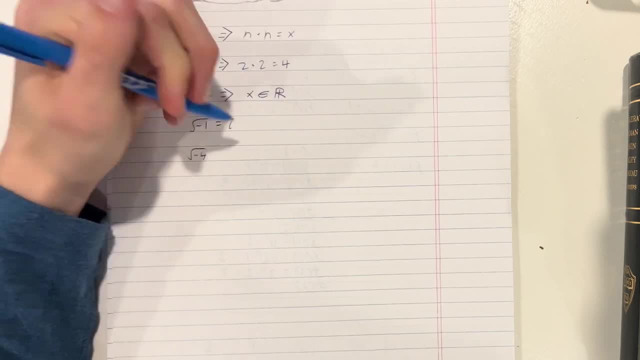 is that there are no real numbers that can be expressed by this. So instead we say that the square root of negative one is i. i is an imaginary number. Now if I ask you again what the square root of negative four is, you could tell me that it is two. i's Alright. 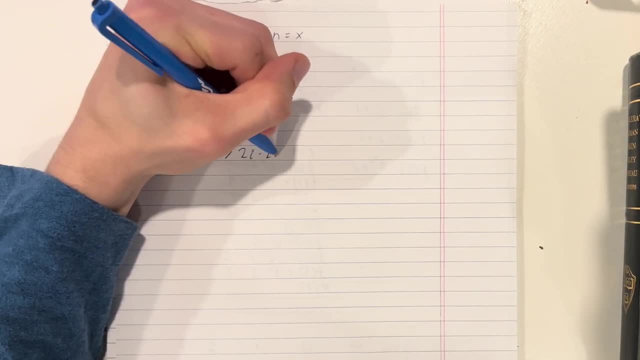 I'm sure somebody will comment on this. I know you were confused about that. It's nothing to worry about… I'm behave capriciousaki. Gracias. i times 2i. To make this a little bit easier to look at, I'll separate out the 2s and the i's. 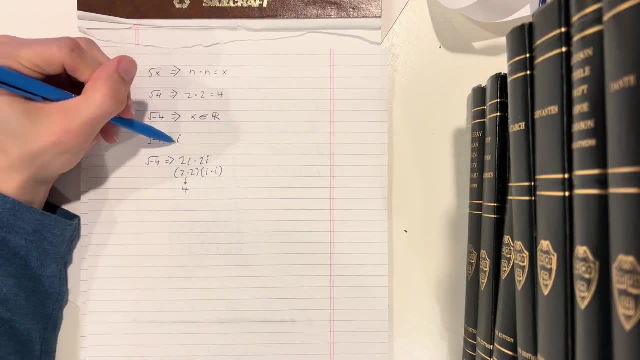 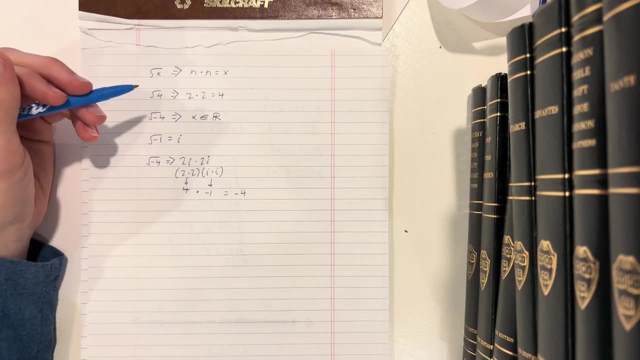 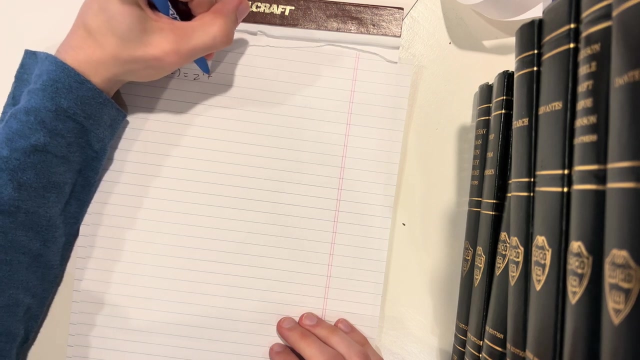 2 times 2 is 4,, of course, and i times i. well, we just described that i times itself is negative 1. This imaginary number i is so crucial in so many mathematical concepts, So Mandelbrot wanted to include imaginary numbers as well in his analysis of this function. Let's try plugging. 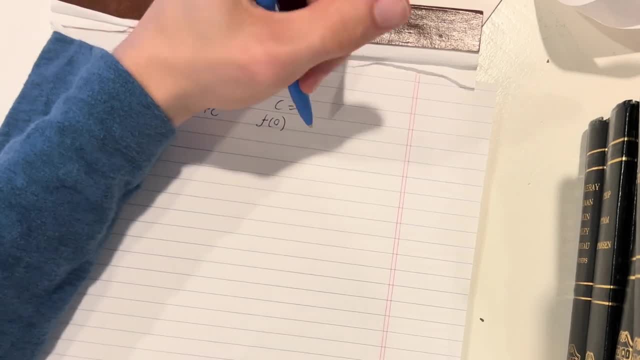 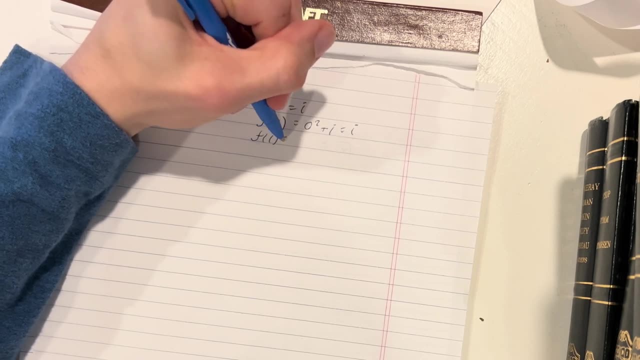 in i for c. Once again, we start with f of 0, and that is equal to 0 squared plus i, which is equal to i. f of i is equal to i squared plus i, and we just defined i squared as negative 1, so this is: 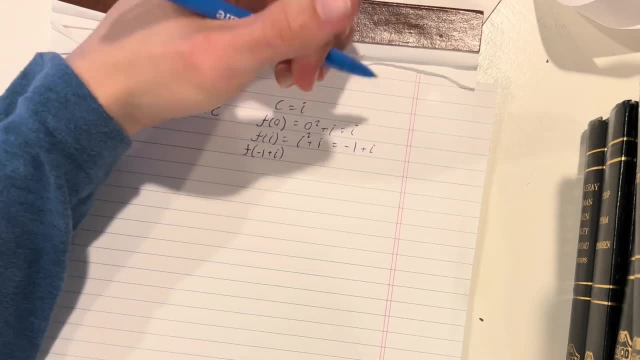 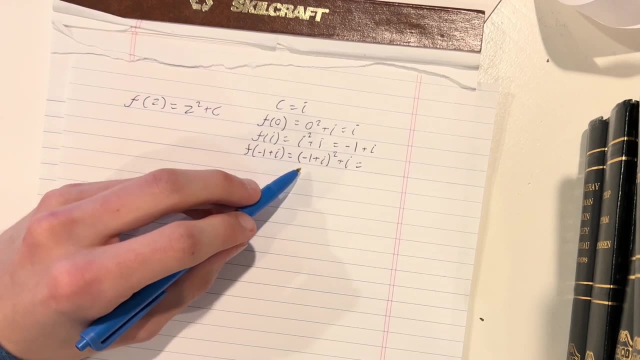 equal to negative 1 plus i. When we get to f of negative 1 plus i, however, things get a bit more complicated. We can't add or subtract real and imaginary numbers, so we'll actually have to bring this down and FOIL it out. 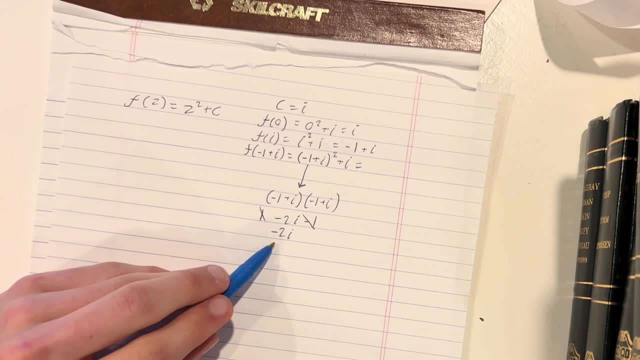 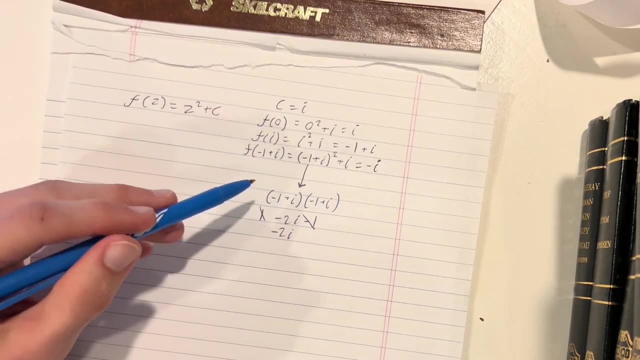 So here we get that negative 1 plus i squared is equal to negative 2i, and negative 2i plus i is negative i Iterations will only get more complicated by hand, so I'll stop here And I'll also tell you that i is actually not included in the Mandelbrot set. This function here will spiral. 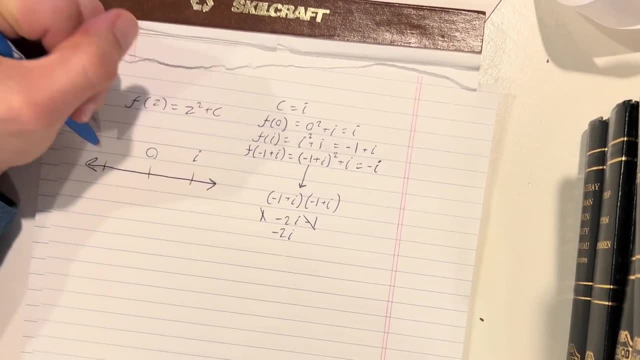 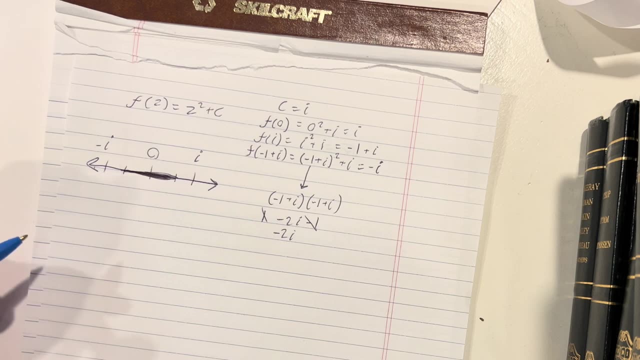 off to infinity. We can set up an imaginary number line here, and I will just tell you that the highest and lowest bounds are roughly 0.6 and negative 0.6.. Many more mathematicians would have stopped there. We've defined it for all of them and we can set up an imaginary number line. 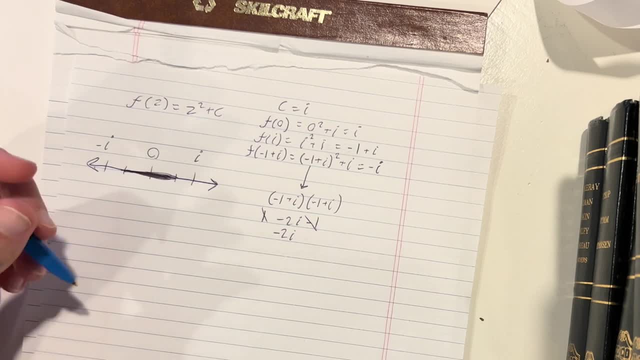 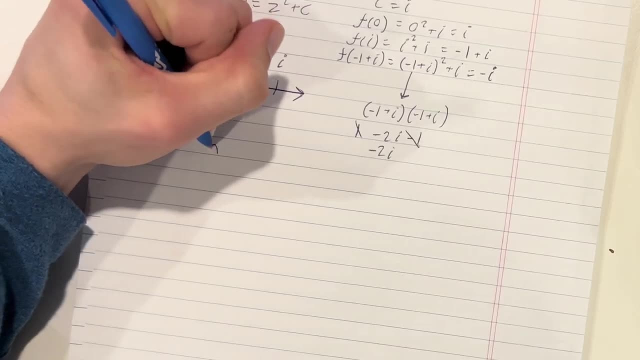 here. When we set up a set of real numbers, we get a set of real numbers, that wealth out of all real numbers and all imaginary numbers. However, in this set there's one more set of real numbers that we haven't looked at yet, And these are complex numbers. Complex numbers have 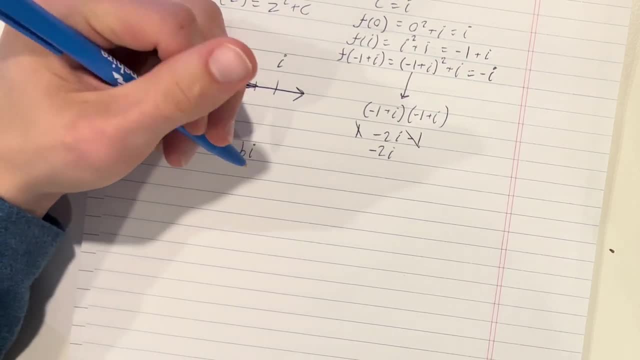 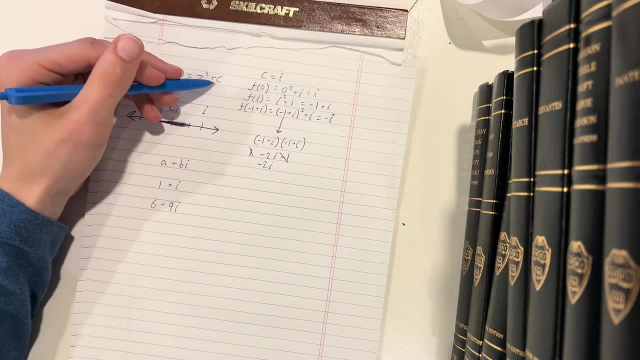 a real and nonreal component. This could be something as easy as one plus i or 6 plus 9i. If we let c be any complex number, then that includes any real, not real or combination of the two. This can be called a complex number. if we let c be complex, The other thing we 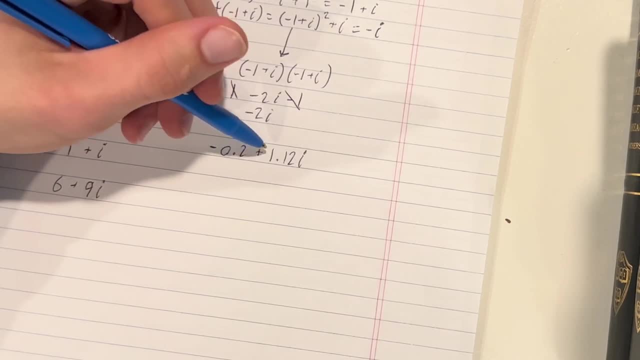 don't have is the real and the nonreal and the nonreal. Someone on reddit told me that your true and false numbers are roughly negative 2i squared and the correct one is only negative negative. 0.2 plus 1.12i is actually included in the Mandelbrot set, but where? 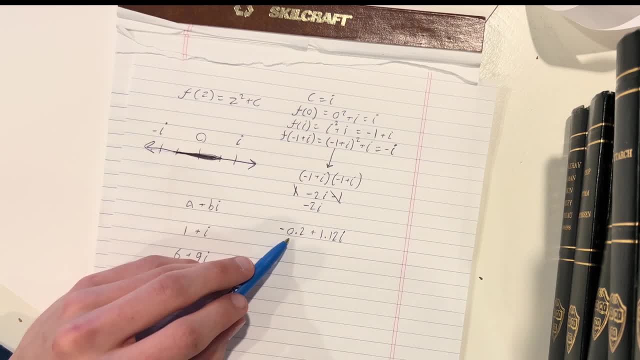 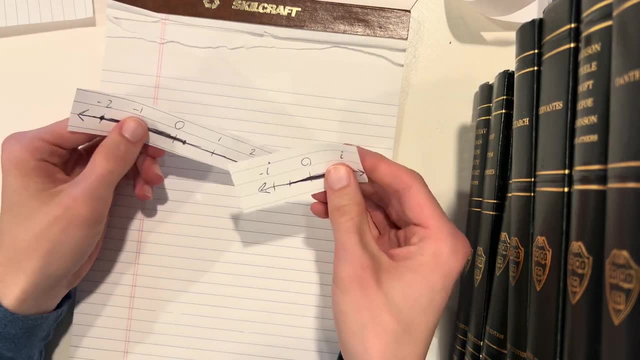 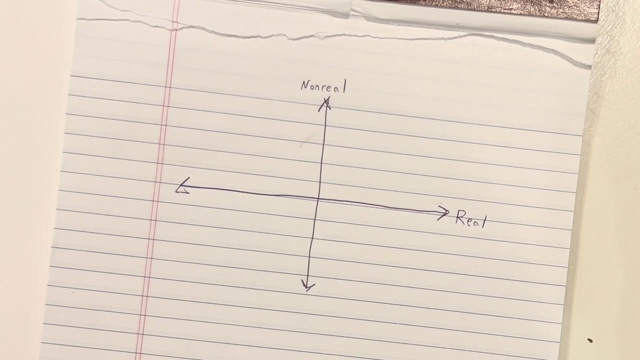 do we put this on the number line? We can't put it here because it also has a negative 0.2.. If only there is some way to view real and non-real numbers at the same time, Introducing the complex plane Real numbers across the horizontal axis. 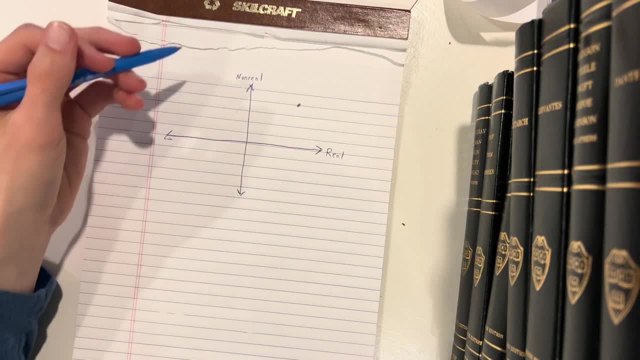 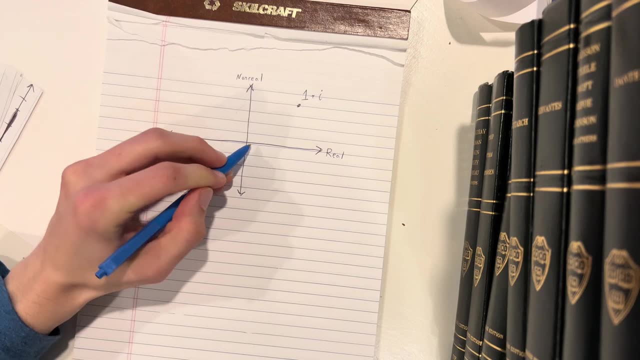 non-real numbers across the vertical axis. I can define any complex number I want by simply placing a point. This could be something like 1 plus i, since we move out one real number and also up i non-real numbers. Finally, we have the. 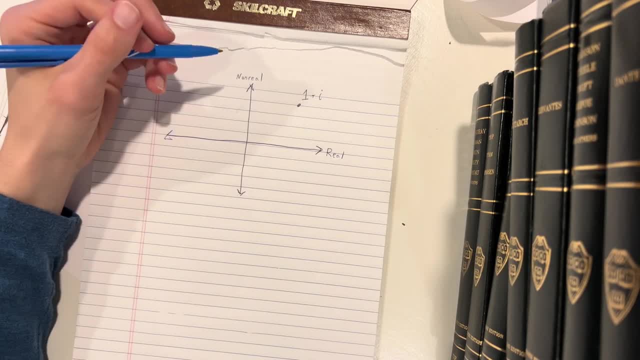 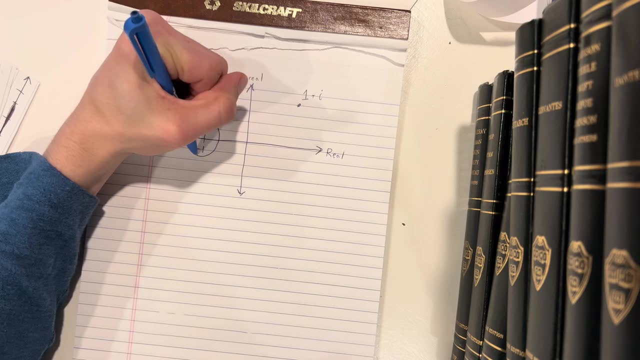 tools we need to graph the Mandelbrot set. This is actually just the set of all. c's such that it does not spiral off into infinity. The Mandelbrot set is a fractal so I can't possibly draw all of it here, but there are several.